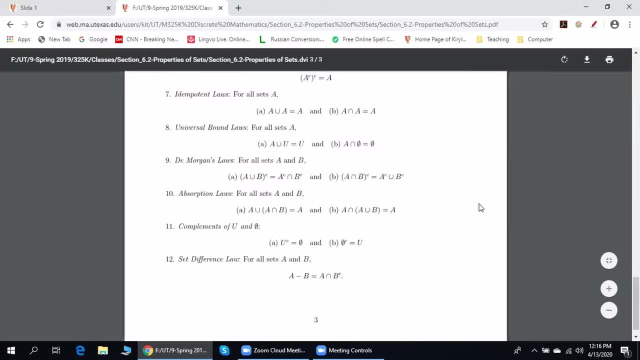 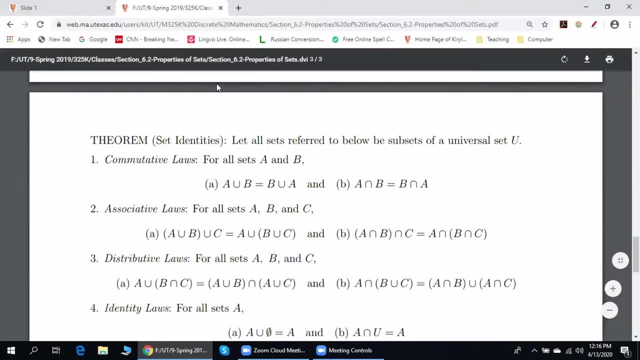 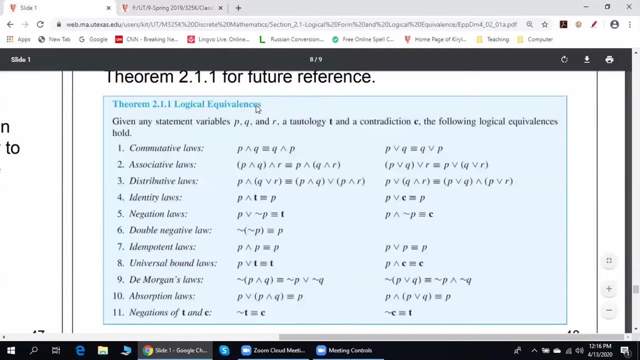 Section 6.2. This one. So please take a look. We have some similarities between logical equivalences and set identities. In both cases we have commutative laws. In both cases we have associative laws. In both cases we have distributive laws. 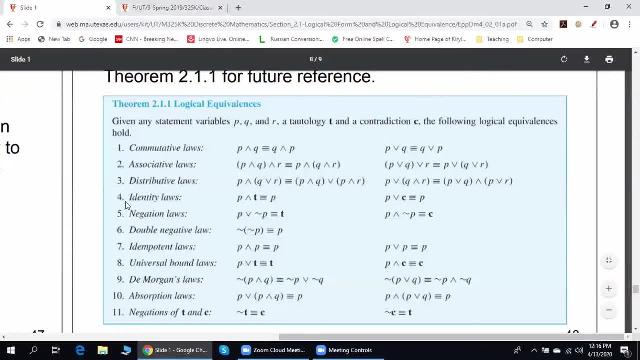 Then please take a look. In both cases we have identity laws. But now be careful. Going back to logical equivalences, Identical laws are: if we consider p and tautology, we get p. If we start with p or contradiction, we get p, again In. 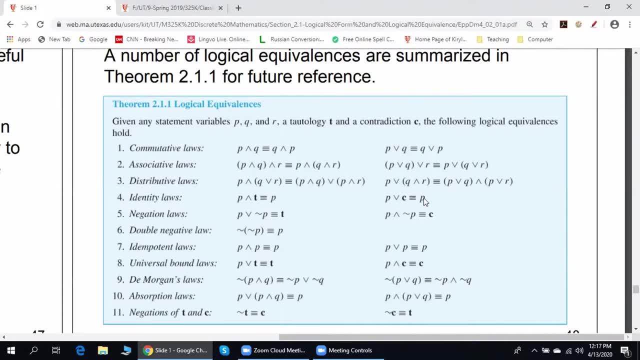 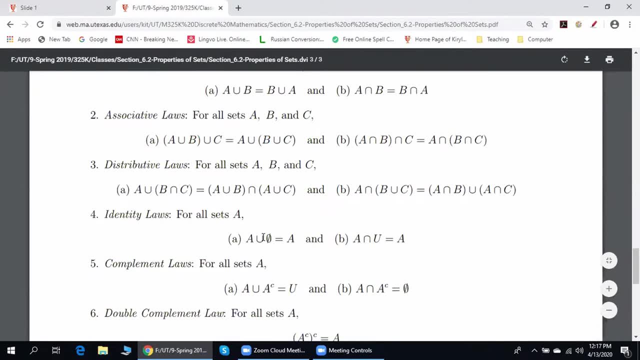 set identities. if we consider a union, the empty set, we get a. If we start with a intersection, the universal set, we get an reset tumor. And then if we include a with these new elements, we get a. If we always have a separate set and we compare it to an alternate set, 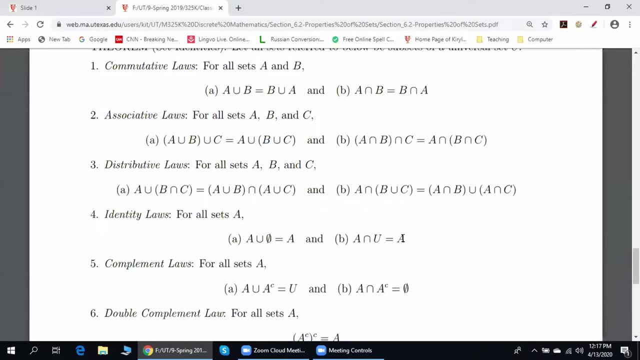 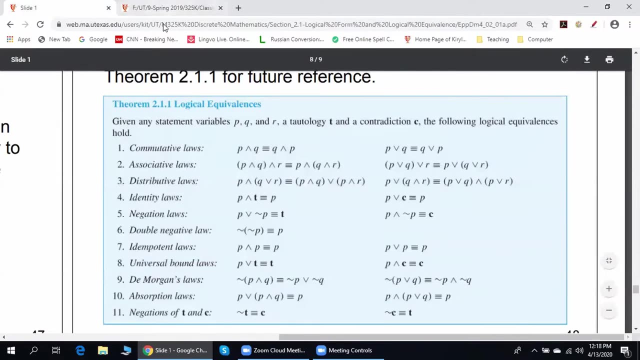 then we get a. If we adopt this method, we get a different set and an integer which is independent and independent. If we nuestrapp», we get a. so it looks like, if you compare this and this, a logical and place a role. 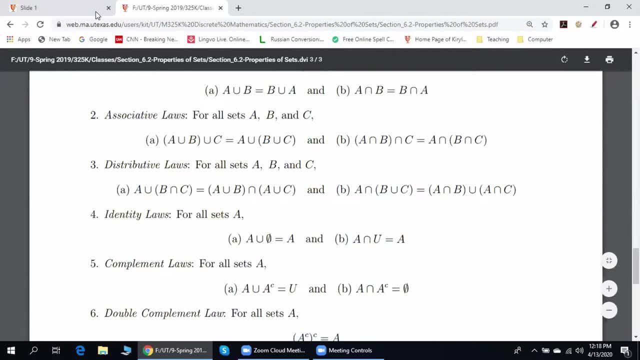 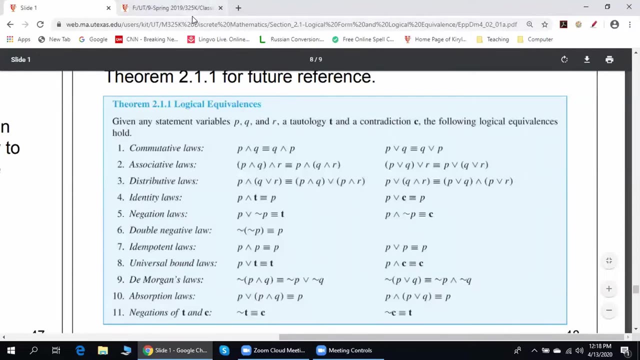 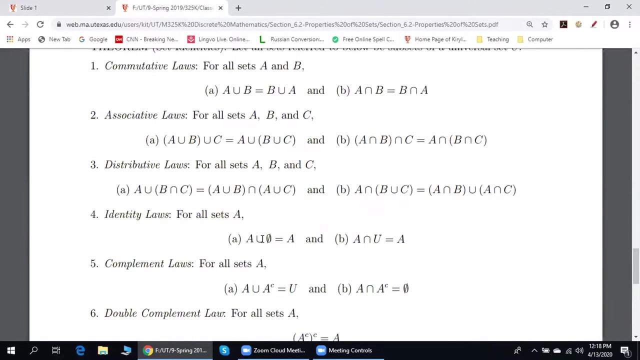 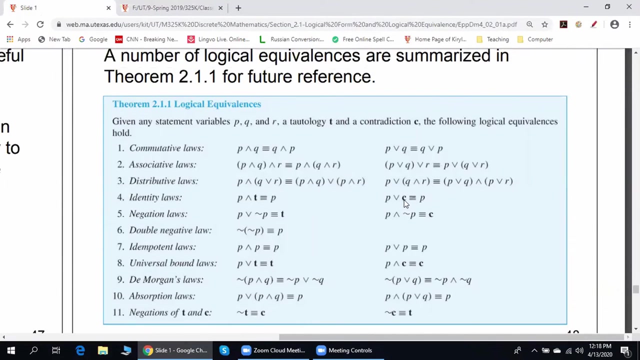 of intersection. tautology plays a role of the universal set. now let us compare this and for a it looks like union plays a role of a logical or and the empty set plays a role of contradiction. please take a look at negation laws. p, or negation of p, is equivalent to tautology. 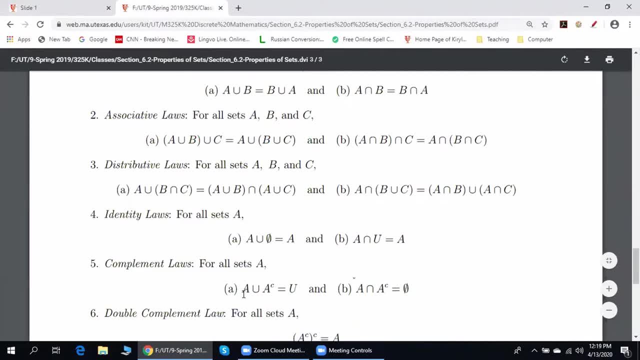 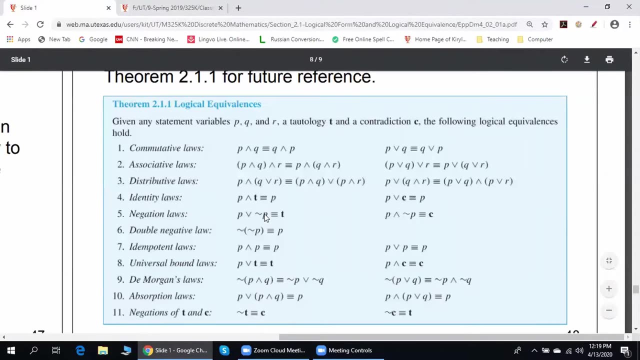 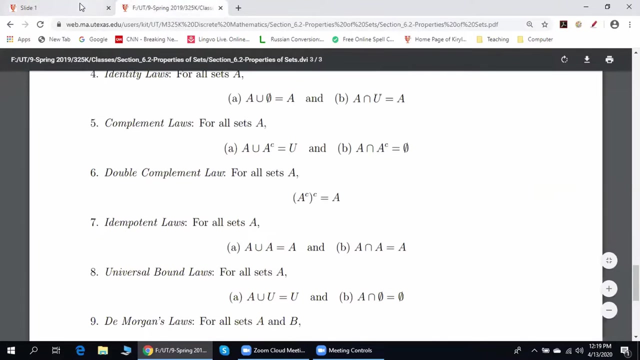 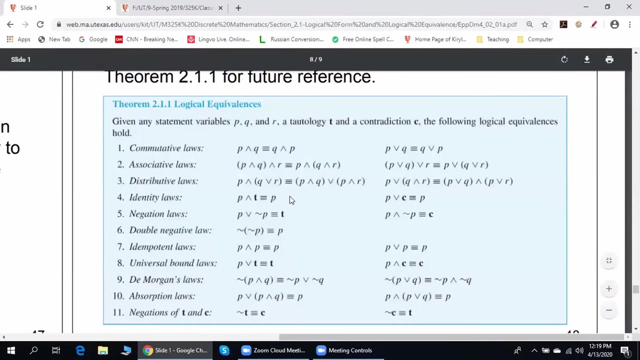 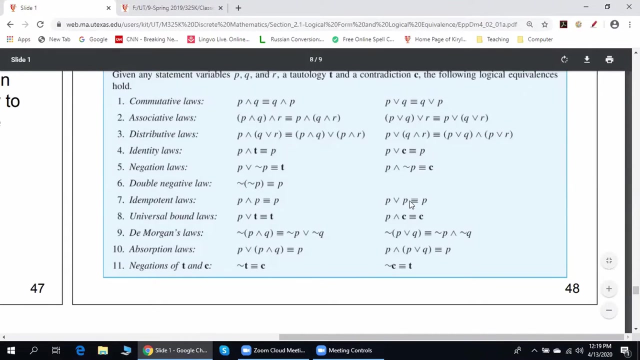 compare with 5a: a union, a complement is equal to the universal set, so it looks like complement plays a role of negation of p. number six: double negation law here. double complement law. number seven: a union, a is a, a intersection, a is a over. here p and p is equivalent to p, p or p is equivalent to p. 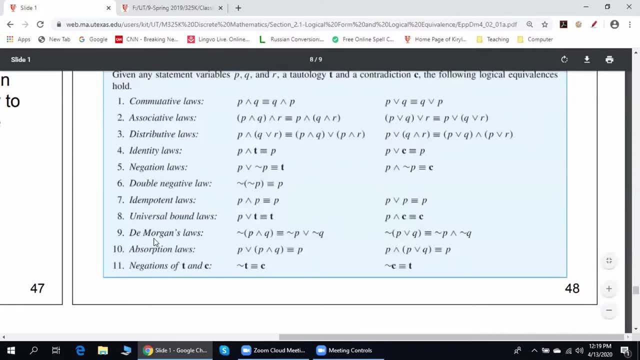 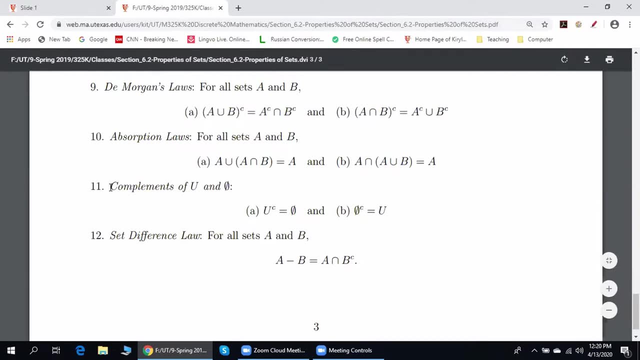 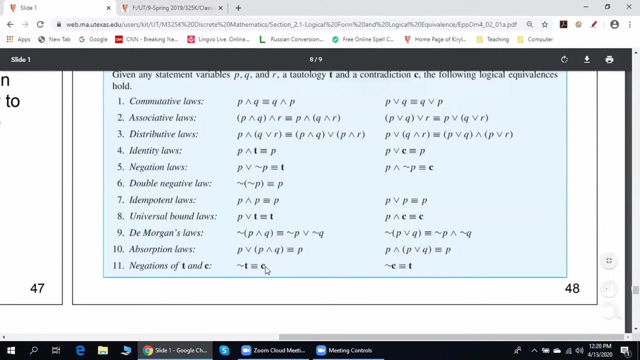 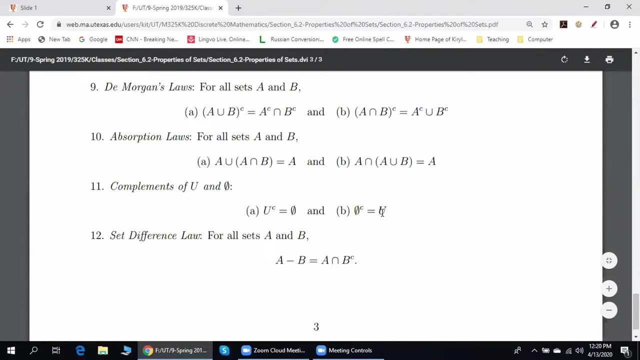 compare also 11 for logical identities and 11 for set identities, complement of the universal set. so for legs a: here a set is equivalent to set and instead of är being adjustment of provided by empty set, the total set is the empty set over. here negation of tautology is equivalent to contradiction. 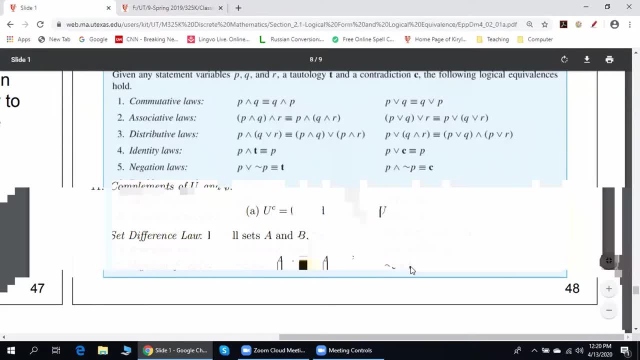 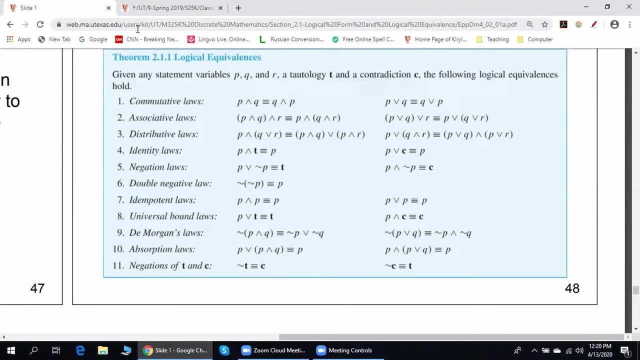 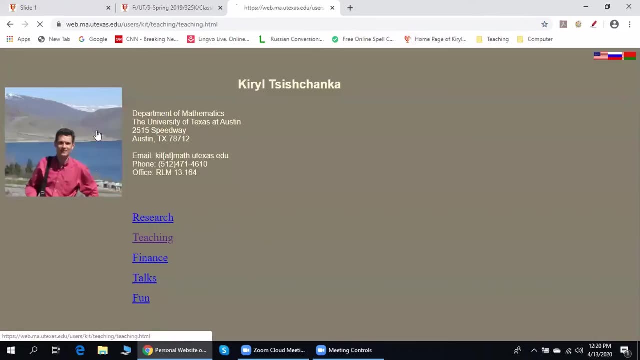 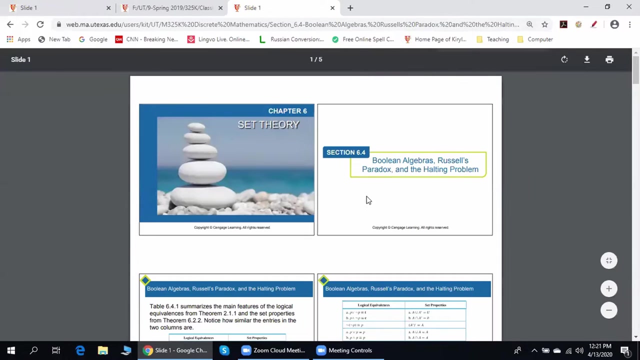 here. complement of the empty set is the universal set over here. negation of contradiction. why do we have these similarities? Is this a coincidence or there is some rationale? It's exactly what we discuss here. Let us talk about so-called Boolean algebras. 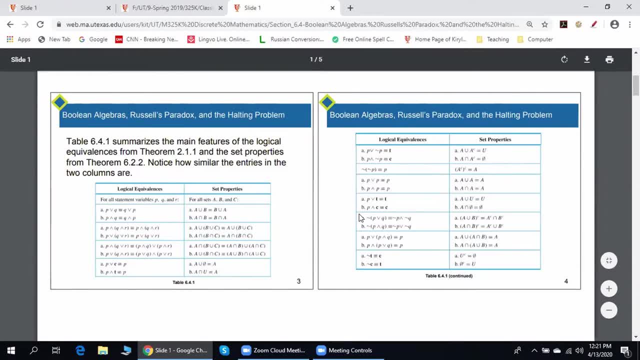 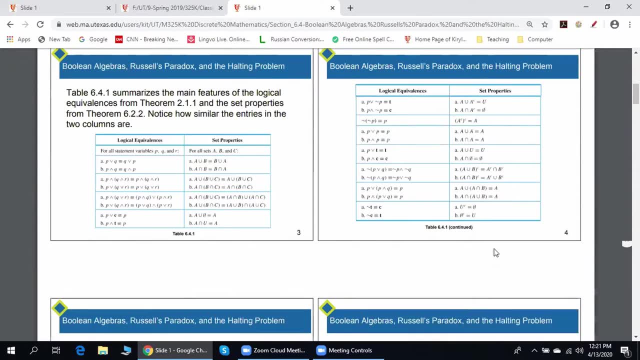 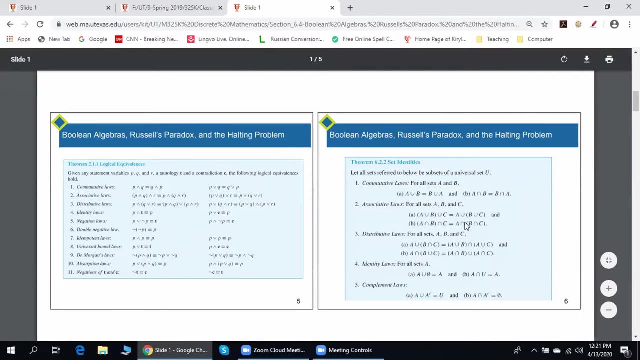 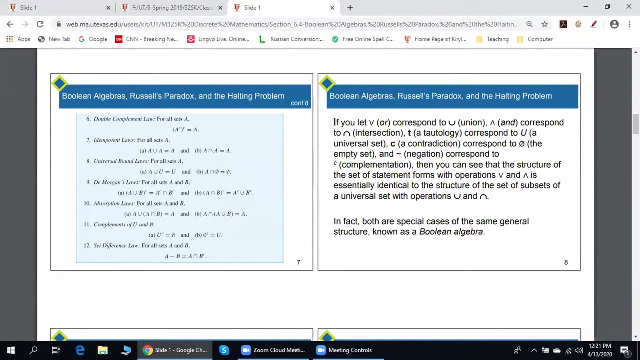 So once again over here we show similarities between logical equivalences and set properties, And here we compare these tables again. So let us read carefully what is written over here. If you let, or correspond to union and correspond to intersection, tautology correspond to the universe. 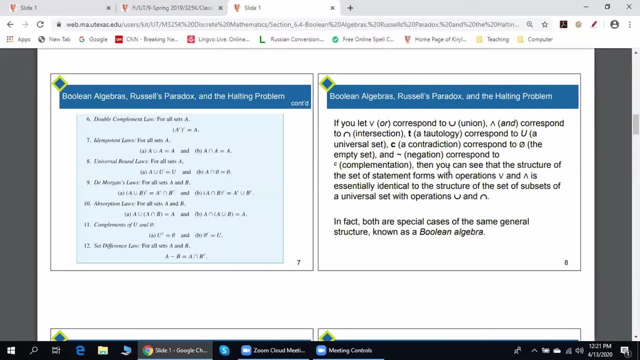 and contradiction correspond to the empty set, negation correspond to complement. Then you can see that the structure of the set of statement forms with operations or, and is essentially identical to the structure of the set of subsets of the universal set with operations, union and intersection. 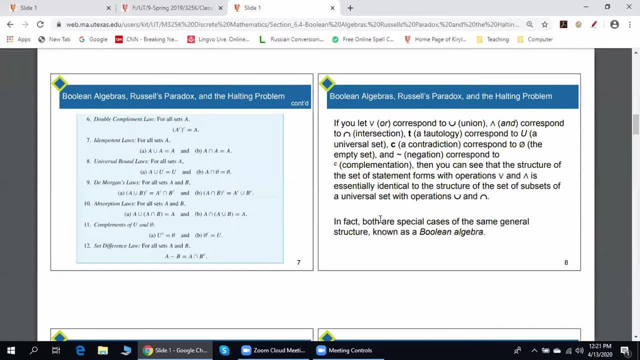 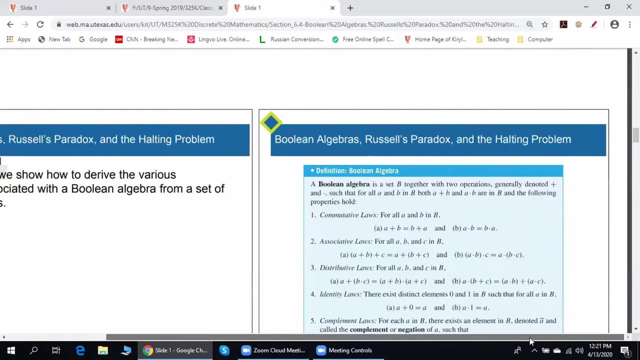 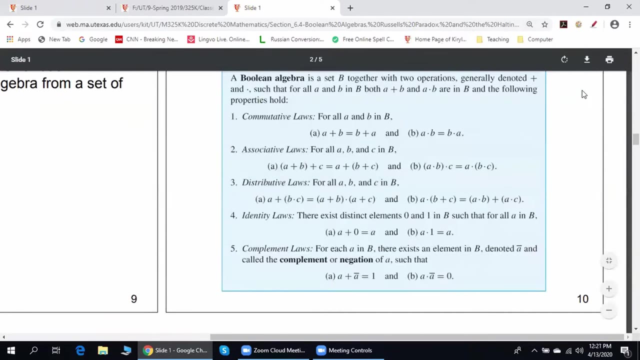 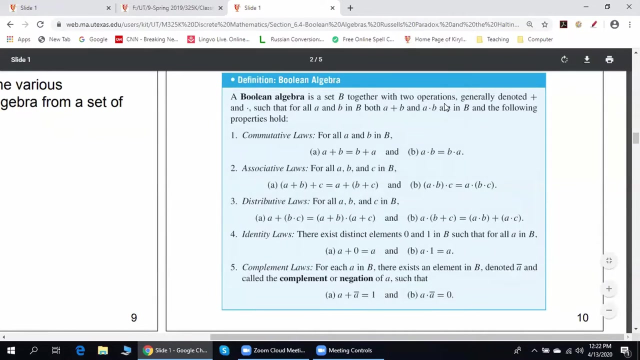 In fact, both are special cases of the same general structure known as a Boolean algebra. Here is what we mean by Boolean algebra. Please take a look at this. A Boolean algebra is a set B together with two operations denoted by plus and times. 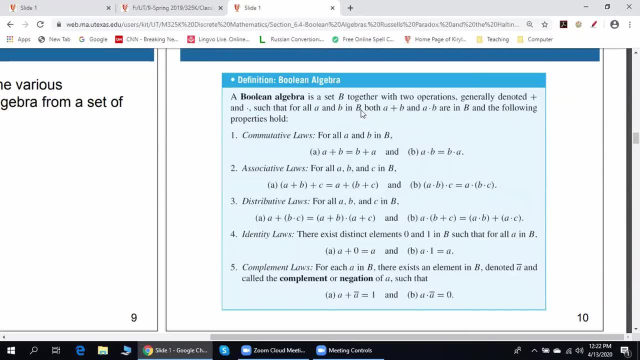 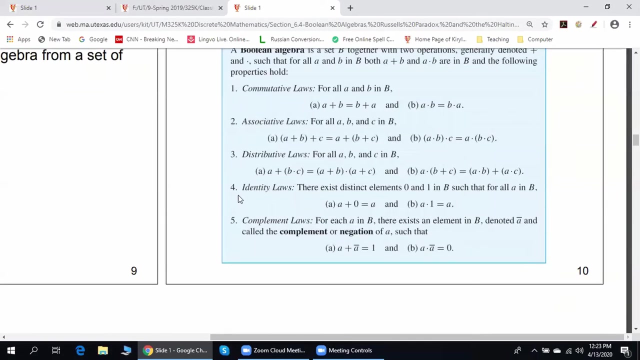 such that for all a and b in B, both a plus b and a times b, are defined and the following properties hold: Number one: commutative laws. Number two: associative laws. Number three: distributive laws, Identity laws, Complement laws. 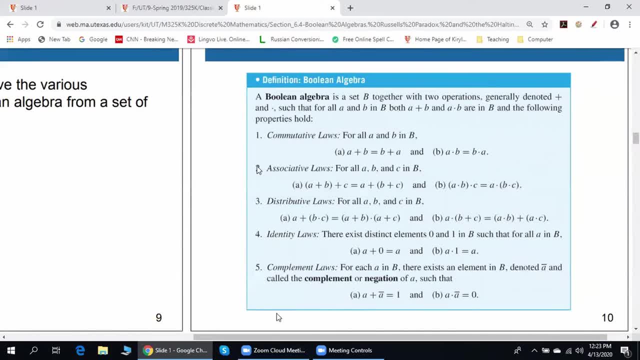 So here we have five laws. May I ask you a question: If we compare plus here and logical operations, what do you think Plus is or or? and Is plus or Plus or times And Times? and If you compare plus and times with set operations? 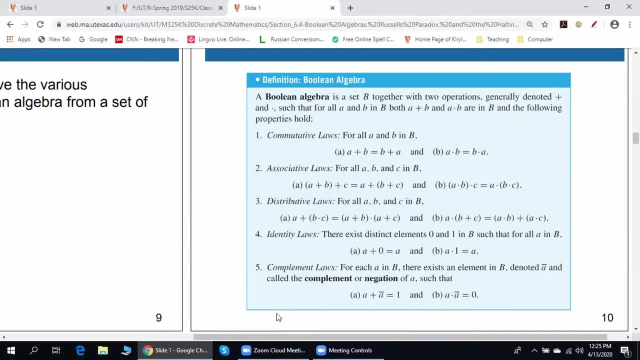 plus is union or intersection. It makes sense that plus would be union, but I don't see how multiplication would be intersection. So question is: how come that multiplication is intersection? What's the problem? I guess the way we're taught multiplication is that it's kind of like adding several times. 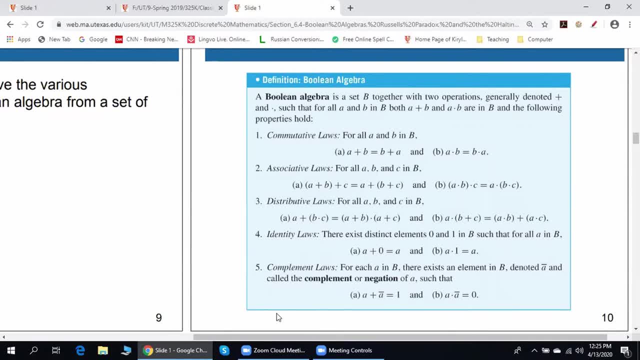 No, no, no. Look, David, it's a very good point. So forget words addition and multiplication. Call plus: operation number one. Call times- operation number two. Now let me restate my question. What do you think? Operation number one? 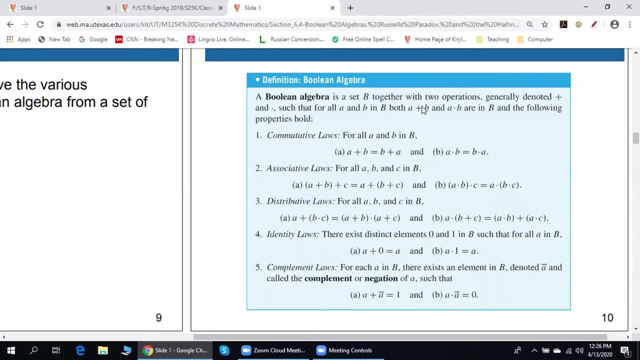 talking about set identities. is it union or intersection? It's union in set Union, Operation number two: is it union or intersection? Intersection, Intersection. May I ask a question? This symbol zero in sets means what? No? 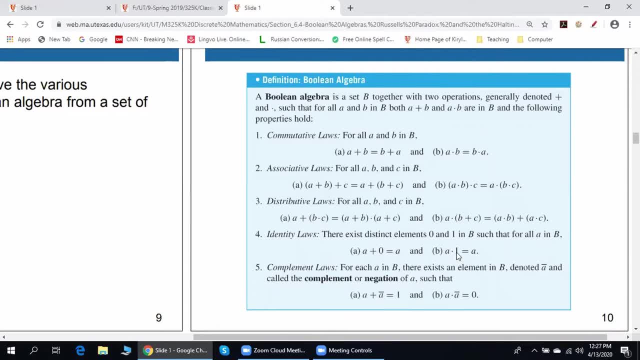 Null set. How about this symbol? one in sets In existing set, Universal set: Yes. So now think about identity loss. A plus zero is equal to A. In sets means the following: A set, A union, The empty set. 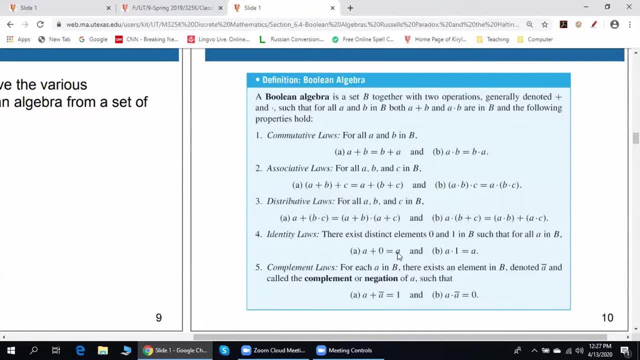 is equal to set A. Yes, Talking about 4B, Can you translate 4B into the language of sets? The intersection of A and the universal set is A. The intersection of A and the universal set is A. It's making sense now, I see it. 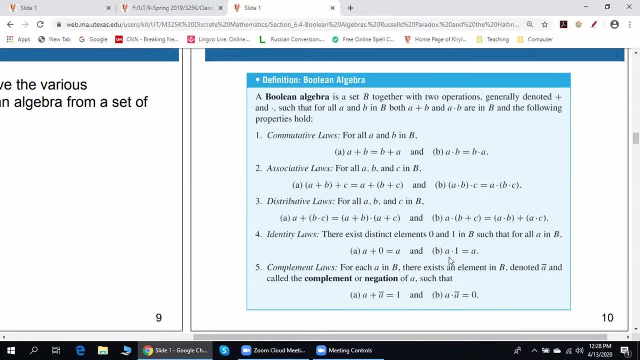 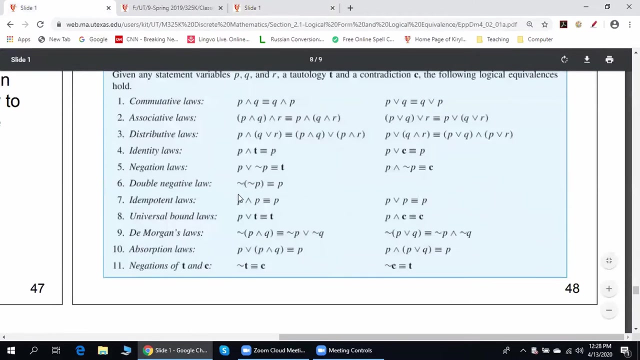 You see it now. Yes, I see it now. Talking about logical operations. Can you translate this and this into the language of logic? A or contradiction is A. A or contradiction is A. Let us go back to this: P or contradiction is P. 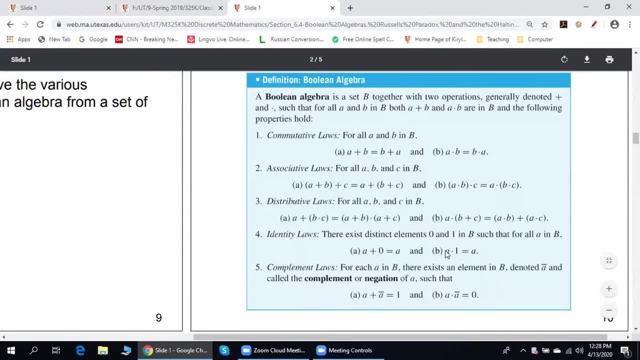 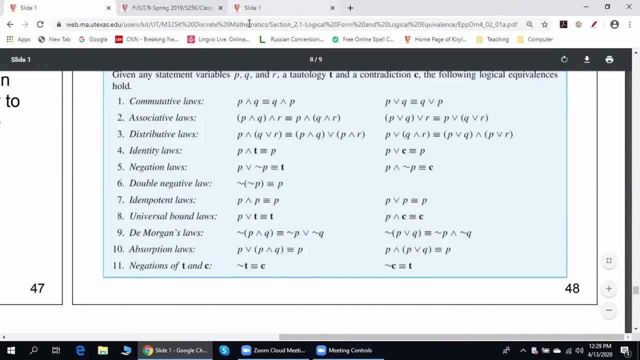 Correct? Yes, How about this? That would be A and tautology is equal to A. P and tautology is equivalent to P. Correct? Yes, It's exactly what is written here: P and tautology is equivalent to P. 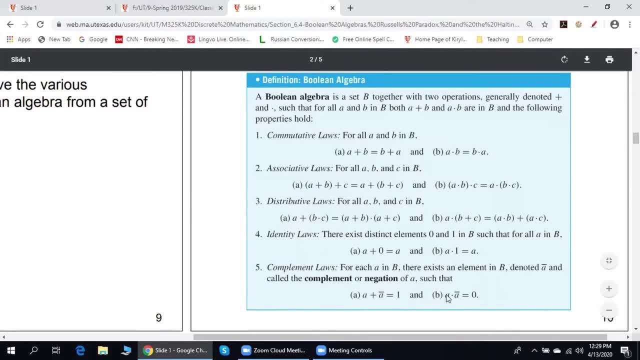 How about this In sets, four sets. Can you translate this into the language of sets? And A bar is the compliments or negation? Say it again. I was really looking for the definition of A bar. So that would mean in set notation. 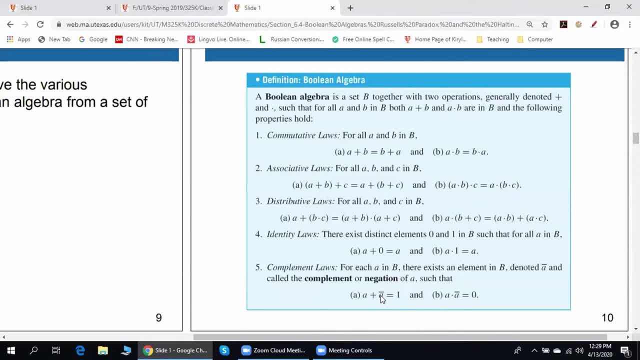 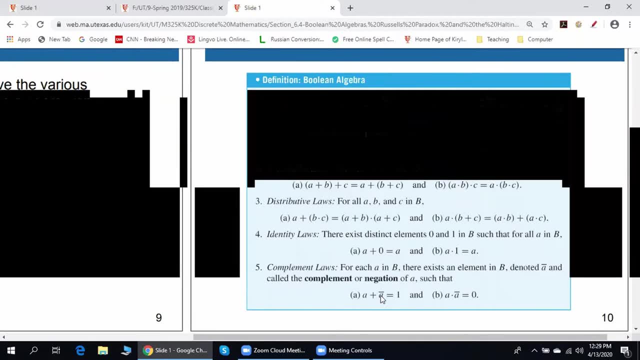 that's the union of A and A. compliments is the universal sets, Right, Exactly. Talking about sets, A bar means compliment. Talking about logic, A bar means what? Oh, in logic, A bar is Negation of A Negation, absolutely. 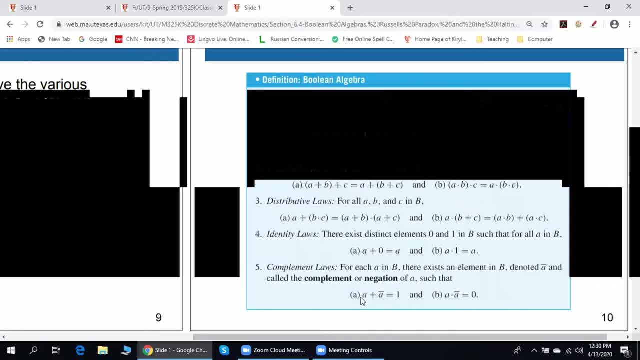 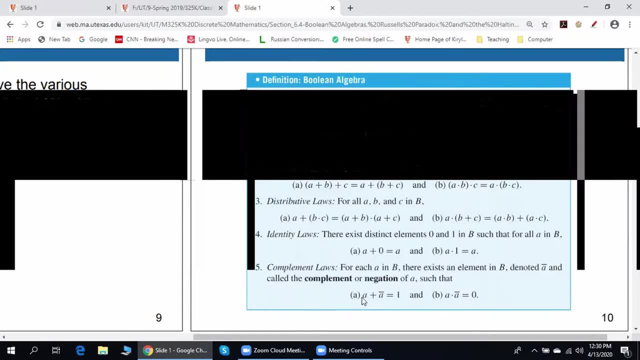 So, going back to sets, 5A means what What? A means what, 5A for sets means what? Just the set A in B. So left-hand side is what? A union, Oh A union, A compliments. A compliment is equal to. 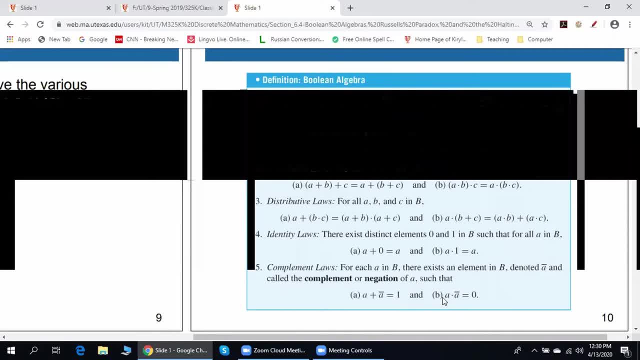 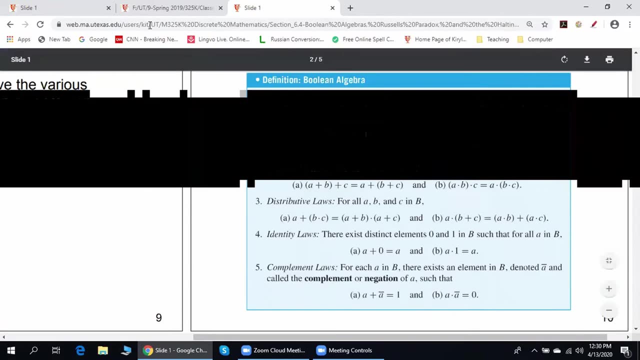 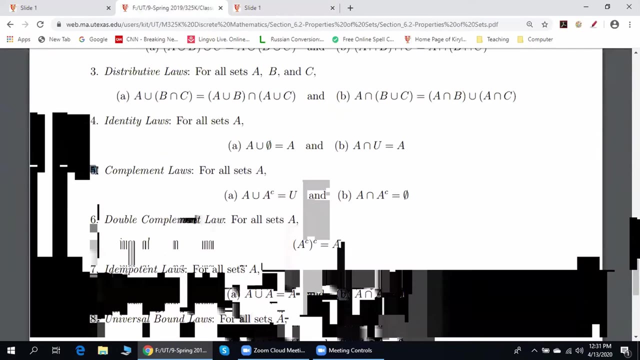 The universal set. The universal set 5B. The intersection of A and A compliments is the null set. The intersection of A and A compliments is the null set. It's exactly what we see here. Number five: A union, A compliment is universal. 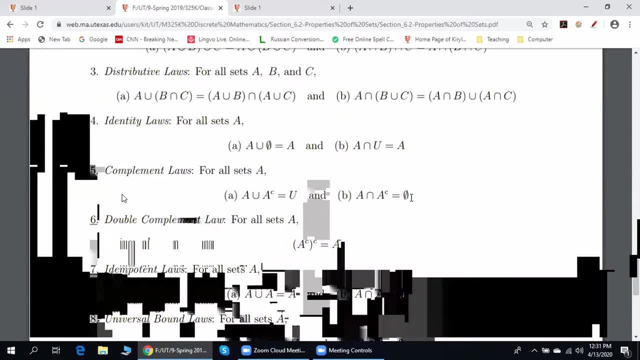 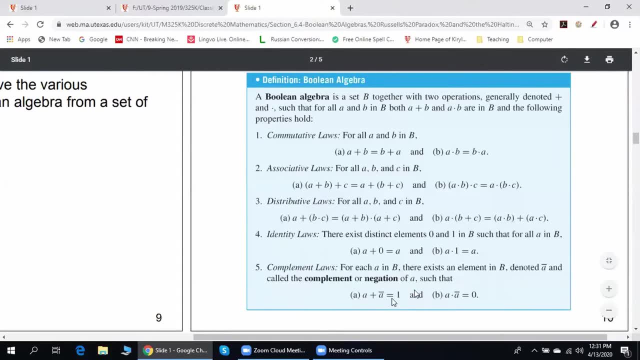 A intersection, A compliment is the empty set. Now, talking about logic, 5A means what? In logic that would mean A or A negation is equal to true. So let us be a little bit more precise: P or negation of P is equivalent. 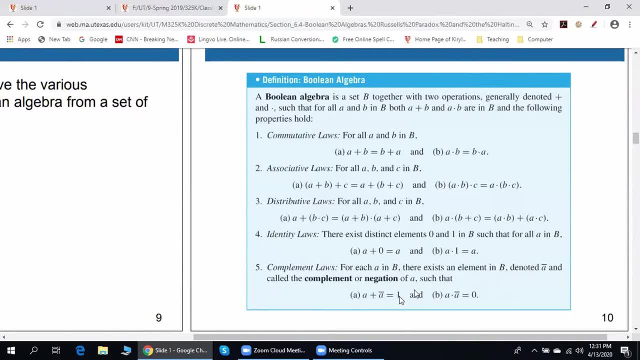 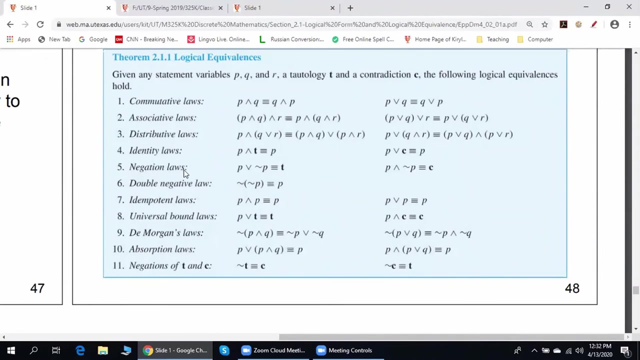 It's equivalent to tautology. To tautology Talking about 5B, That would be P and negation P is equivalent to contradiction. P and negation P is equivalent to contradiction. It's exactly what we have here: Negation laws. 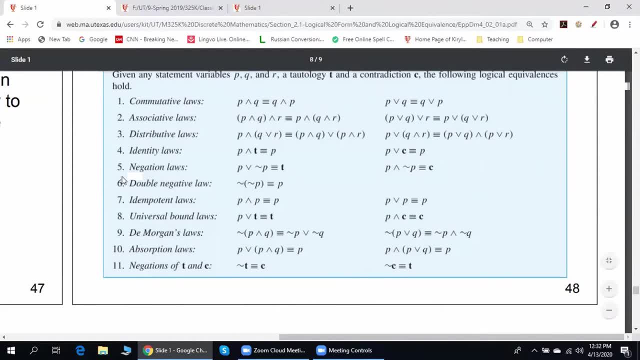 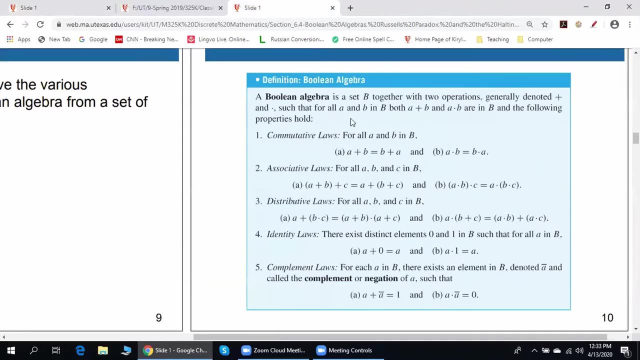 So, once again, 5 here is equivalent to 5 here. P or negation of P is equivalent to tautology P and negation of P is equivalent to contradiction. Guys, any questions here? Can you give an example of what if A pick A, A being a number, what A compliment would be? 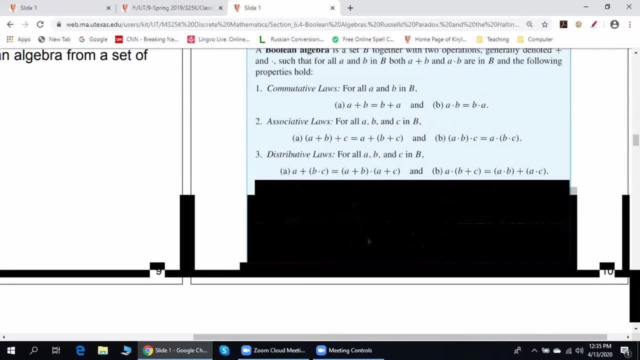 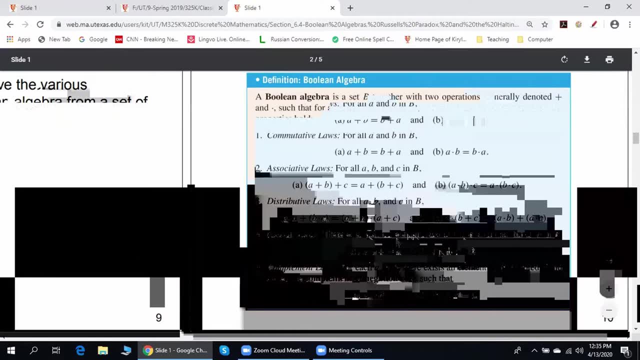 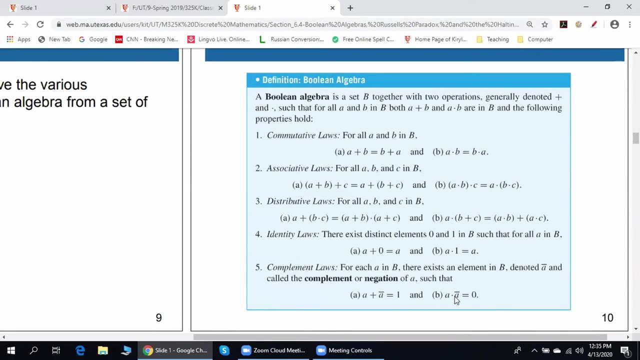 I'm just trying to visualize how A plus A compliment is equal to 1.. And what does 1 mean in this case? So, depending on the situation, 0 and 1 and bar mean different things. For example, talking about sets, by 1,, we mean a universal set. 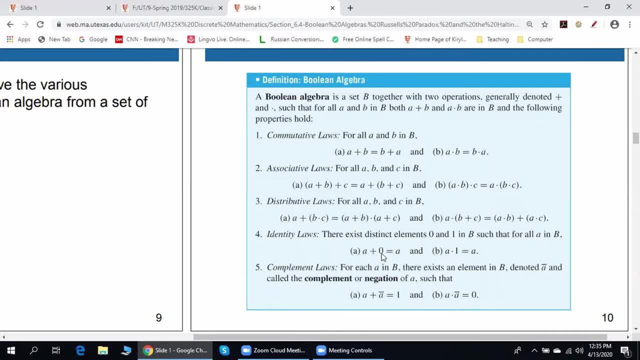 By 0, we mean the empty set. Okay, Okay, By bar, we mean compliment, So this is not really 1.. This is not really 0. Right, Okay, Like these rules in our context. Okay, I understand. 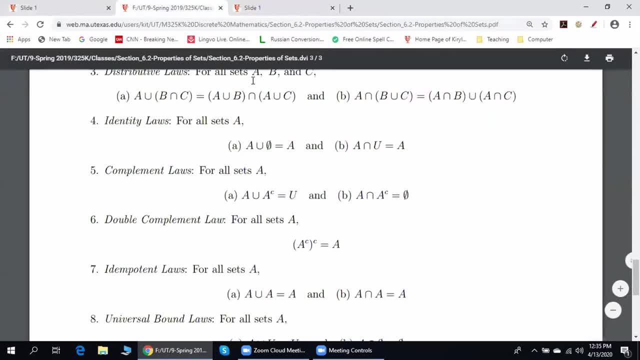 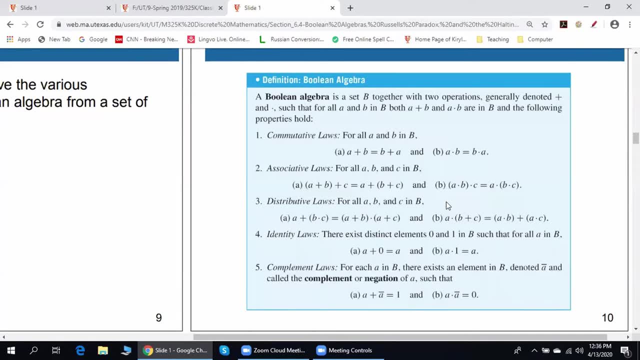 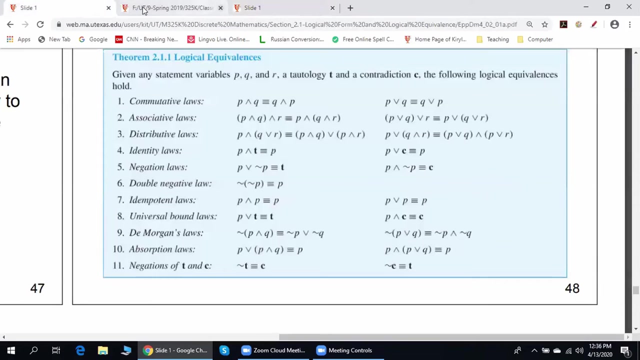 You either logic or sets, So little a and little b are both examples of sets. Is that what you're saying? Yes, Okay, Gotcha. So applying these rules to sets, A, B, C are sets. Okay, If we want to apply these rules to logic, A, B, C will be statement variables. 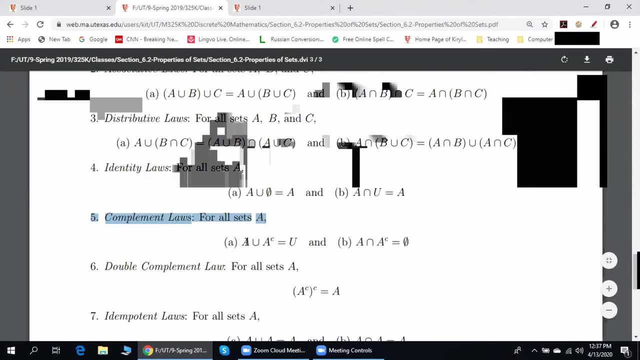 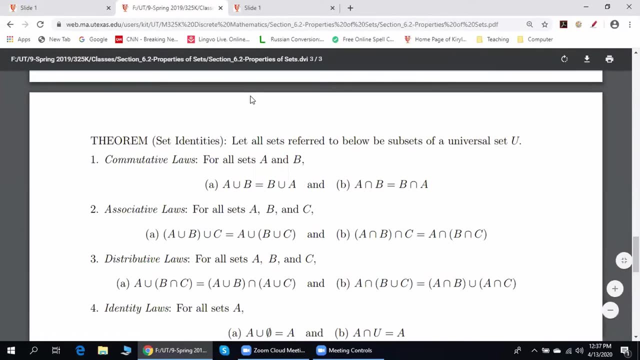 Does this make sense? I guess so, but why are you doing it in terms of Boolean algebra, Like? what's the reasoning for learning, for doing Boolean algebra, then? in this case, The reason is the following: We see similarities between logical equivalences and set identities. 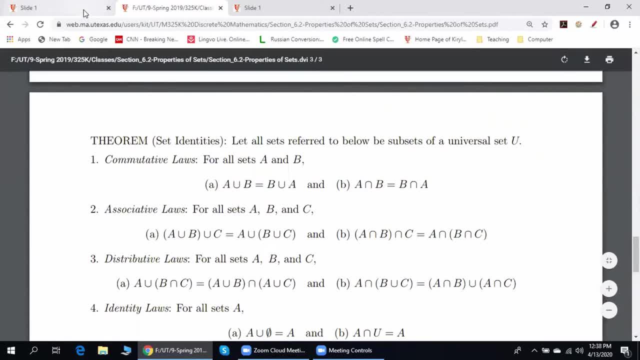 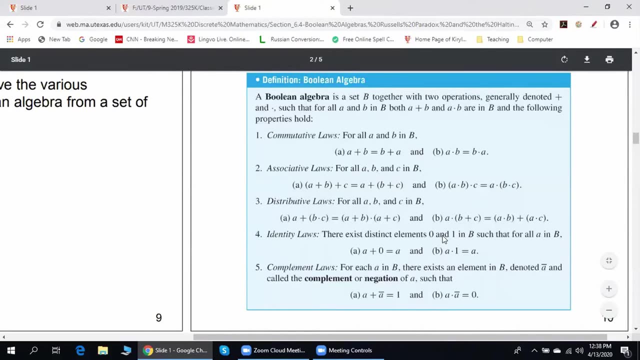 We're trying to explain why logical equivalences look like set identities. Okay, So what do they call 1, 0 in Boolean algebra? Is that just? They don't, They wouldn't call it. We call it. So in Boolean algebra they call it 0 and 1.. 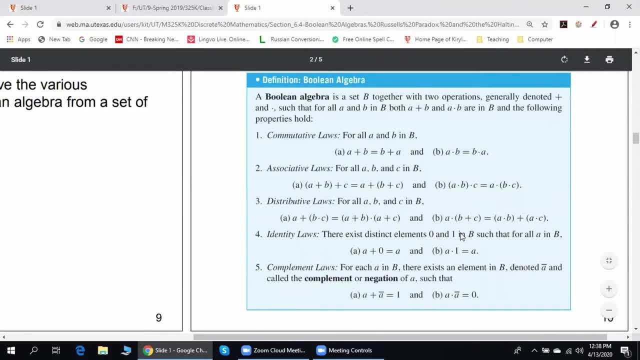 Okay, 0 and 1.. Oh, I guess. Okay, But this is how we call it. You can call this operation plus. You can call this operation times. You can call it, But in particular, plus in Boolean algebra means union in sets. 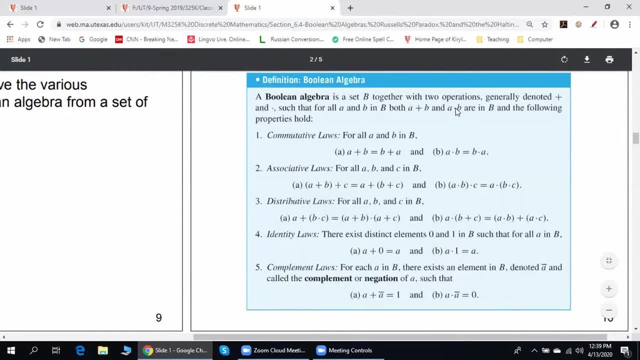 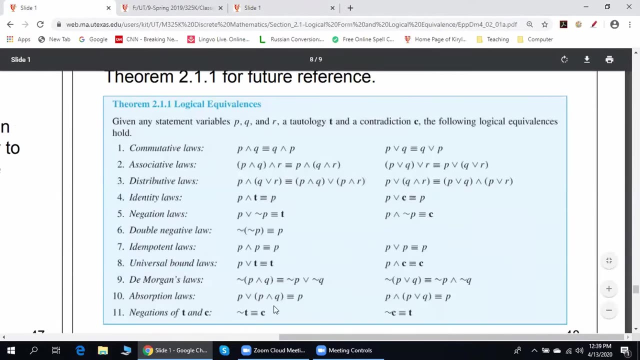 Times in Boolean algebra means intersection in sets. Okay, So 1 and 0, is that the same as true and false Or No, no, no Or just 0 in logic means contradiction. 1 in logic means tautology. 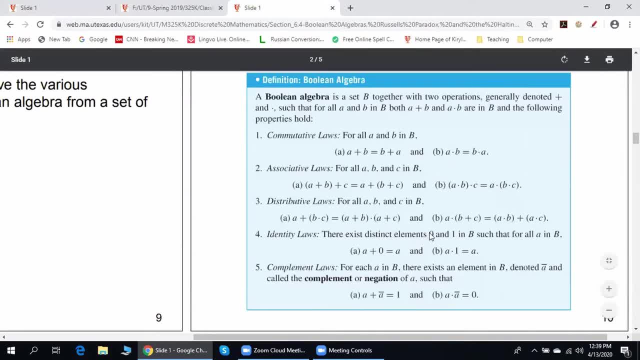 Okay, Okay, I see, I understand. 0 in sets means the empty set, 1 in sets means the universal set. Okay, Does this answer your question? Yeah, yeah, yeah, I got it. Thanks. Now you may ask me a question. 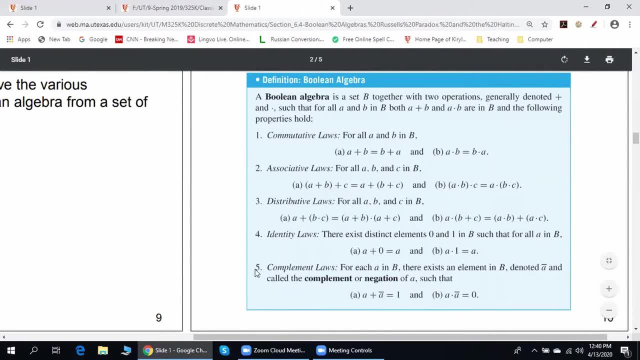 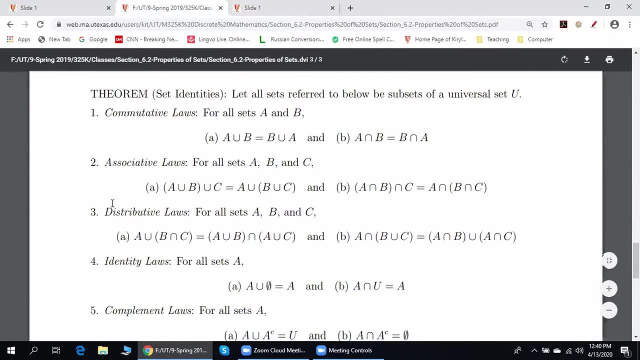 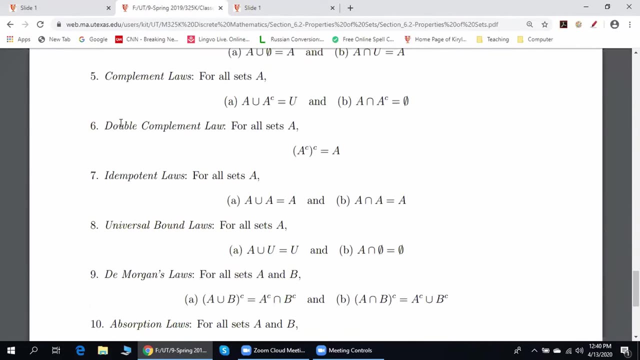 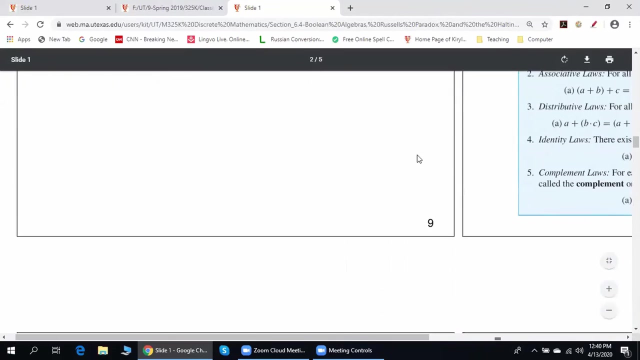 Wait a second. Here we have just five rules, And these five rules correspond to these five rules. How about double complement law, universal bound law, De Morgan's law? The answer is: we can deduce all these laws from these five rules. 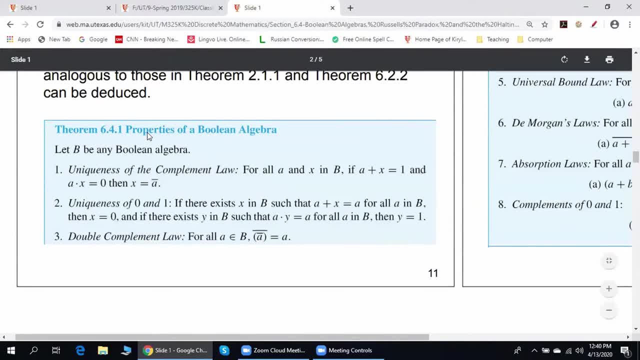 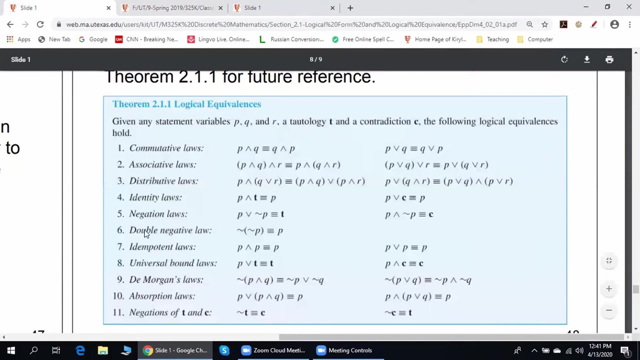 For example. please take a look at this theorem: Uniqueness of the complement law, uniqueness of 0 and 1, double complement law. By the way, double complement law corresponds to double complement law for sets and double negation law in logic. 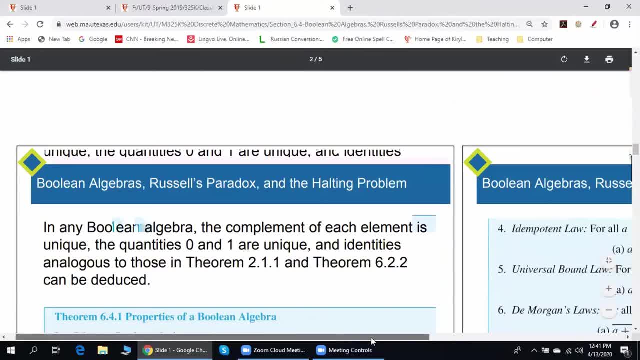 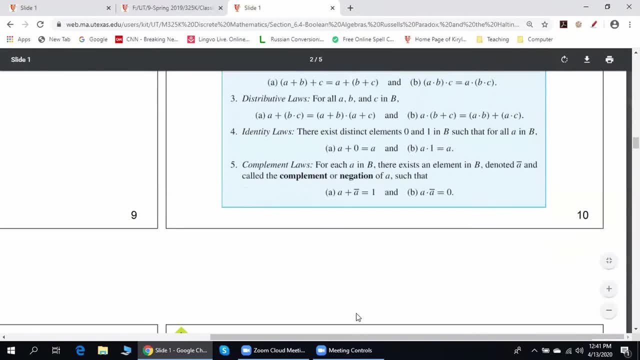 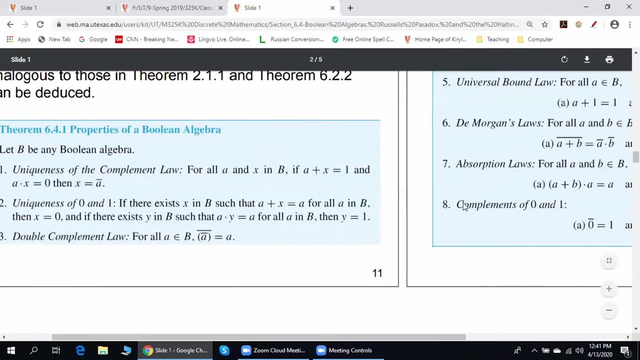 So, in other words, we will use only five rules from this definition in order to deduce the rest. And here we have in this theorem we have eight additional laws, And then the remaining laws in sets, and logic will follow from this. 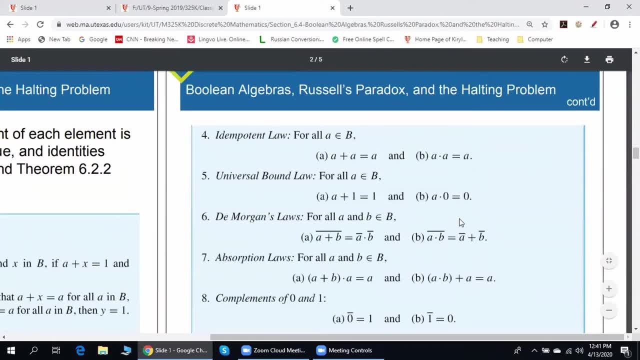 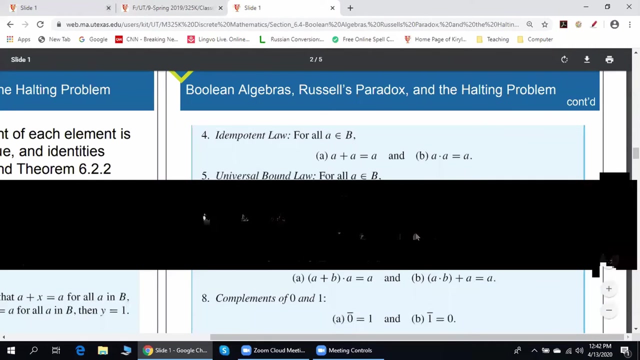 For example De Morgan's law: a plus b bar is a bar times v bar. a b bar is a bar plus b bar. In the language of logic, 6a corresponds to 9b And 6b corresponds to 9a. 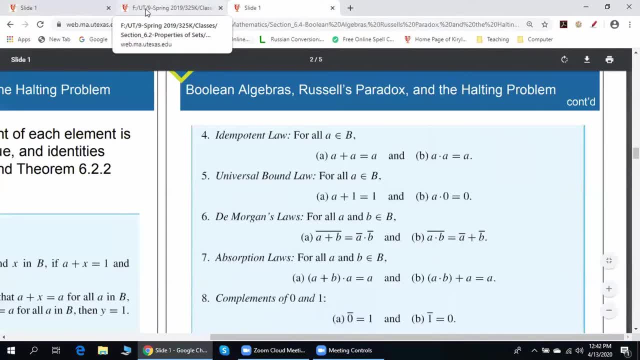 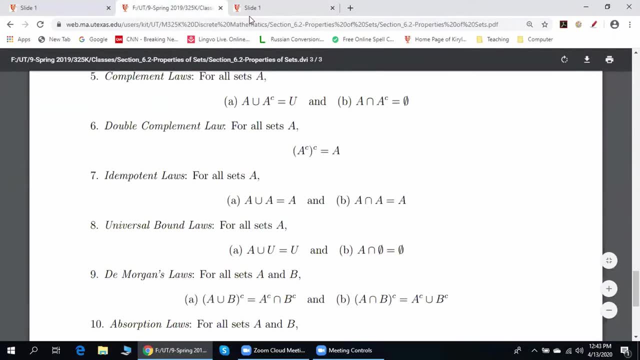 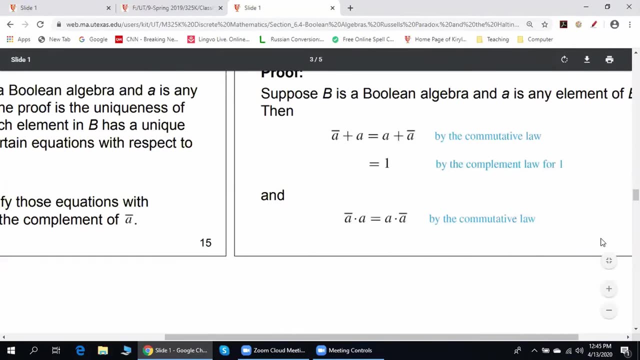 If you compare this with sets and logic, you will see that 6b corresponds to 9a. If you compare this with sets and logic, you will see that 6b corresponds to 9a. If you compare this with set identities, 6a corresponds to 9a and 6b corresponds to 9b. 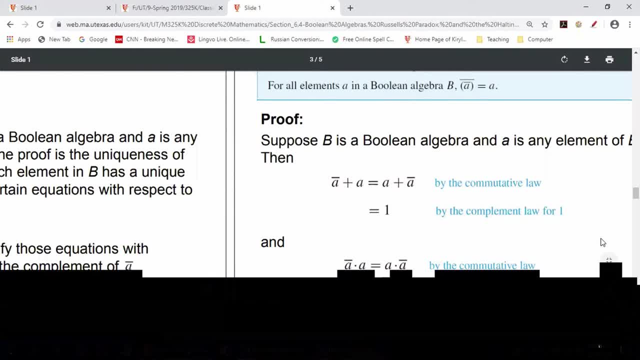 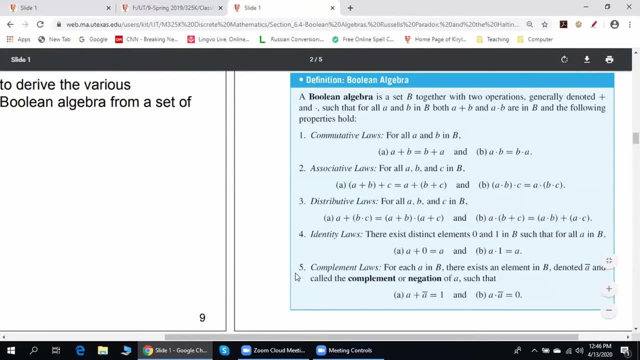 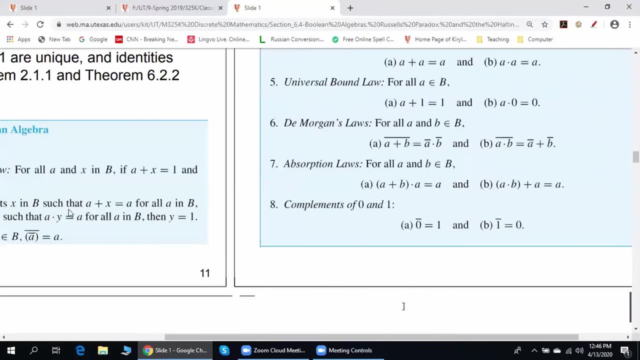 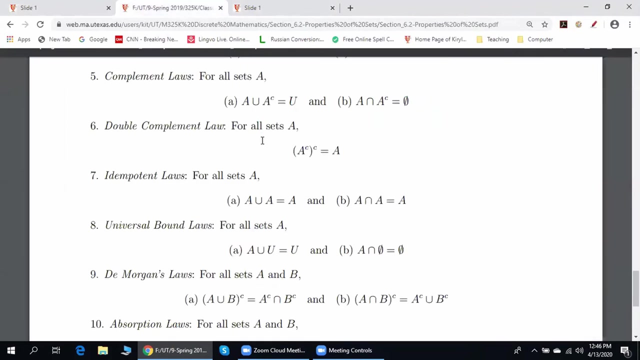 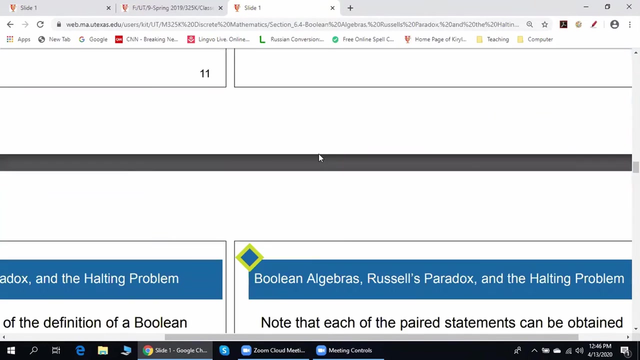 Think about questions. So, once again, what we see in front of us here is definition. We have five basic properties, And then from these five basic properties we deduce the remaining eight, And then the remaining property here and here follow from these eight properties. 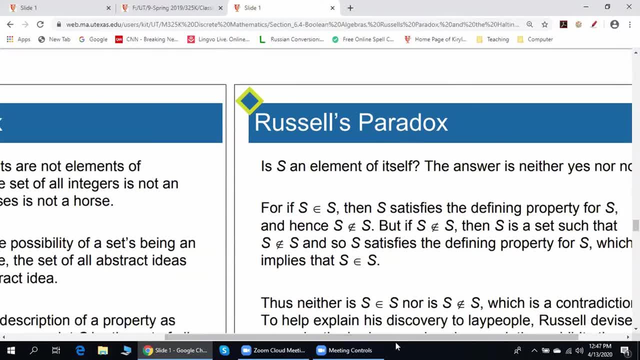 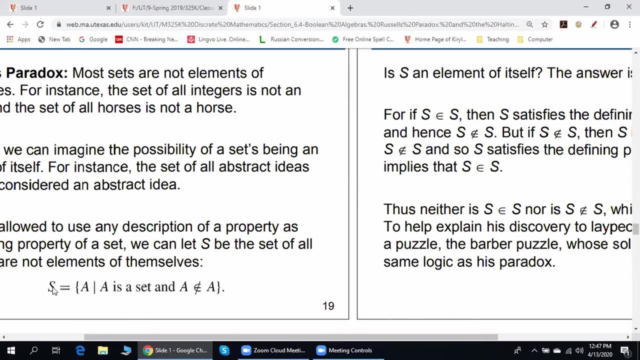 Last thing for today is Russell's paradox. Let us consider the following set S: The set S consists of all sets that are not elements of itself. The set S consists of all sets that are not elements of itself. Question Is: set S an element of itself? 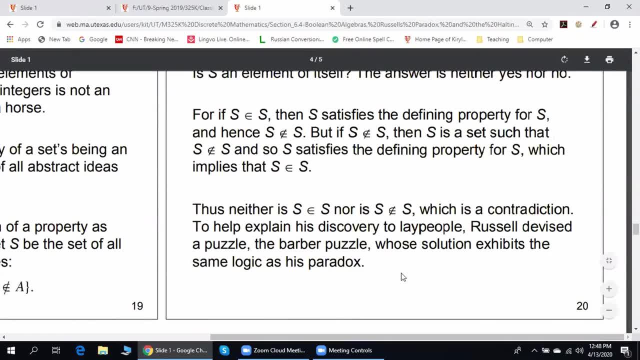 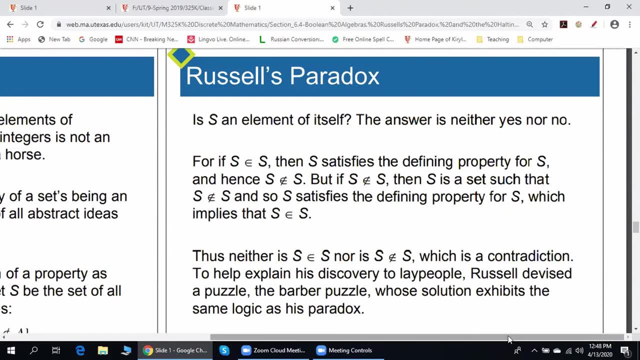 Is set S an element of itself. Unfortunately, we cannot really answer this question. The answer is neither yes nor no, And this is why we call it paradox. And this is why we call it paradox. Here's why. Well, there are two possibilities: S is an element of itself or S is not an element of itself. 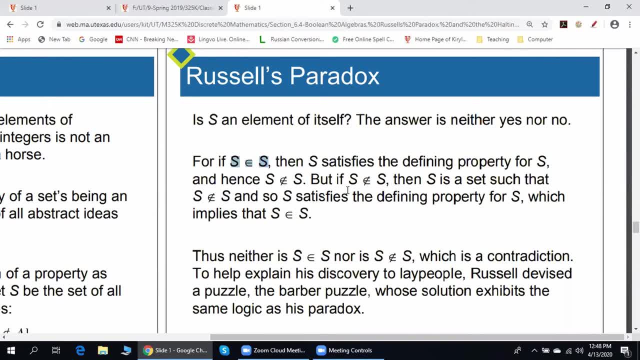 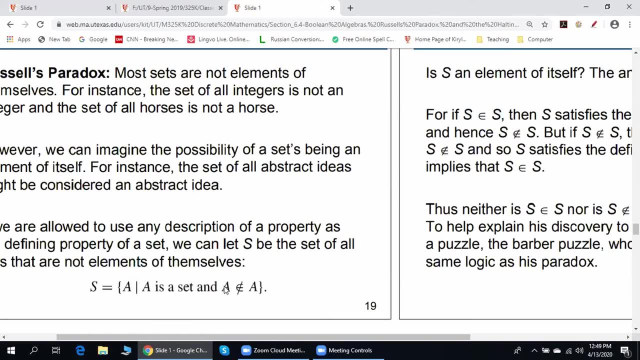 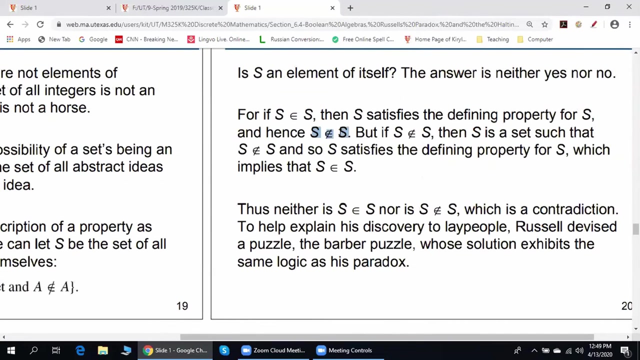 Suppose S is an element of itself. If S is an element of itself, then S does not satisfy this property. Since S does not satisfy this property, S cannot be an element of itself. Therefore, S is not an element of itself and we get a contradiction. If S is an element of itself, S is not an element of itself. 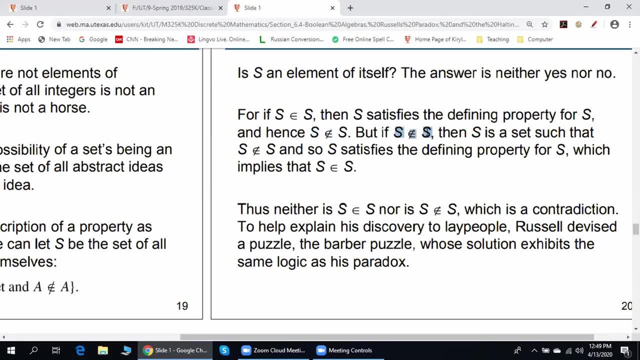 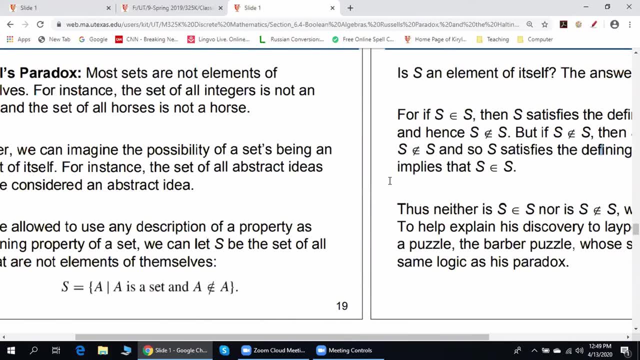 Vice versa. Suppose S is not an element of itself. If S is not an element of itself, then S does satisfy. this property Means S is an element of itself. So if S is not an element of itself, S is an element of itself, and we got a contradiction. 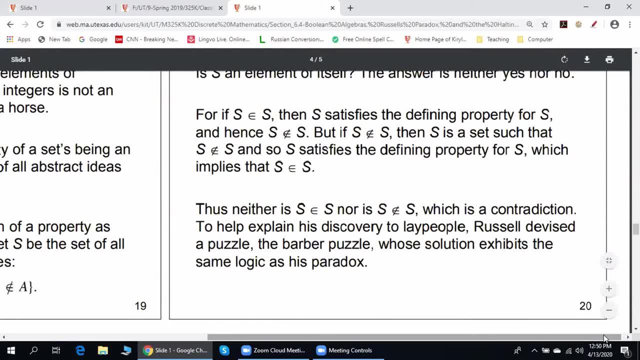 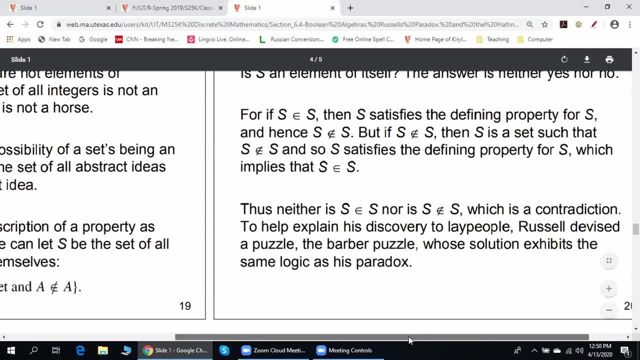 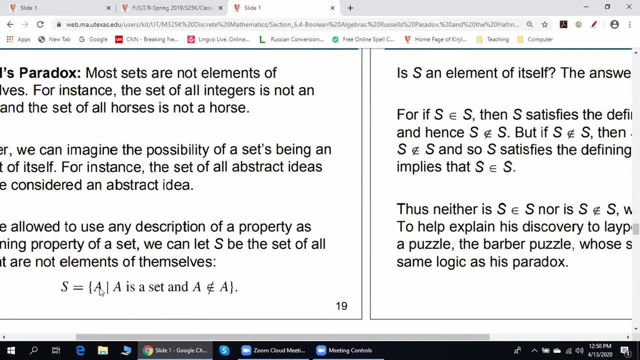 Any questions here? Can you explain this once again? Yes, So set S consists of all sets that satisfy the following property: A is not an element of itself. Now for set S. there are two possibilities. Now for set S, there are two possibilities. 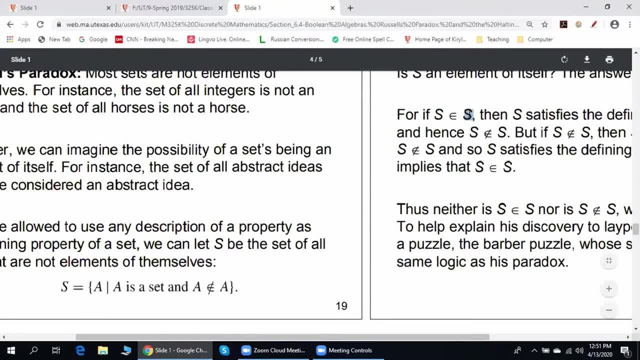 S by itself is an element of itself or S by itself is not an element of itself. Now in both cases we get a contradiction. So case 1. Suppose S is an element of itself. Since S is an element of itself, it does not satisfy this property. 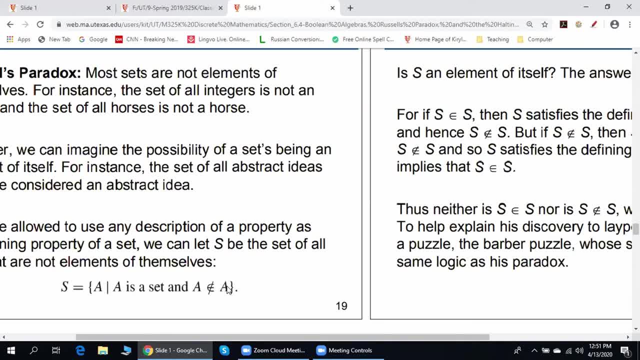 property. Correct, Because S is an element of itself. Here we consider the set of all sets that are not elements of itself. So since S is an element of itself, S is not from this set, Correct? Therefore, S is not an element of itself Because S is not here. 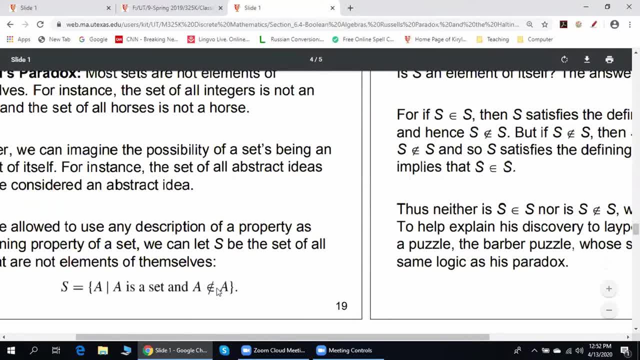 Because if S is here, S is not an element of itself, But S is an element of itself. So S cannot be from here. Since S is not from here, S is not an element of itself. We got a contradiction. We started with the following: 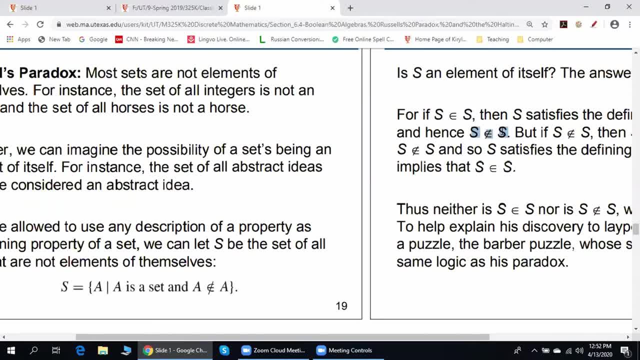 S is an element of itself. S is not an element of itself. We came up with the following contradiction: S is not an element of itself. Does this make sense? Correct? Now case two: Suppose S is not an element of itself. 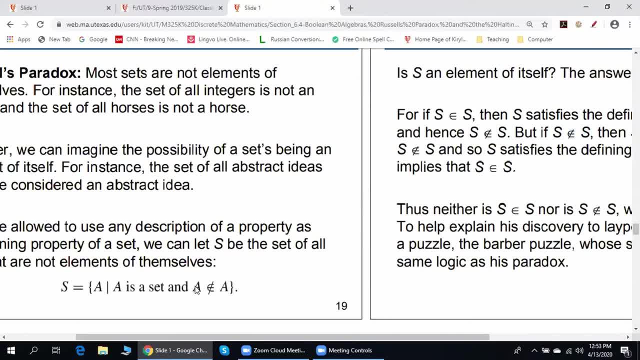 Since S is not an element of itself, it does satisfy this property. Correct? Since S does satisfy this property, S is from here. Since S is from here, S is from itself, Which is exactly what is written here. We got a contradiction. 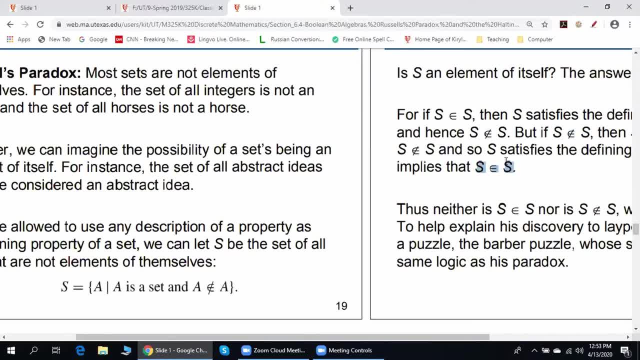 S is not an element of itself and S is an element of itself. In both cases we got a contradiction. Does this answer your question? Yes, So how do you deal with the fact that the statement is either true or false?